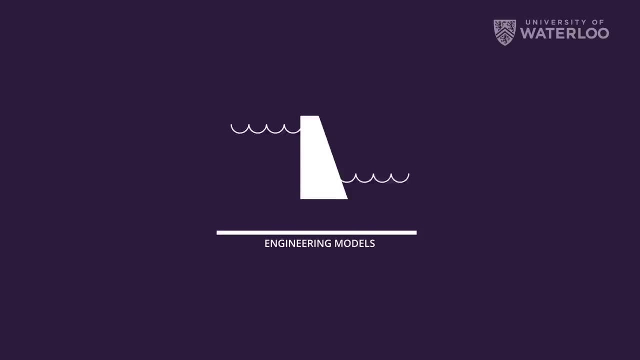 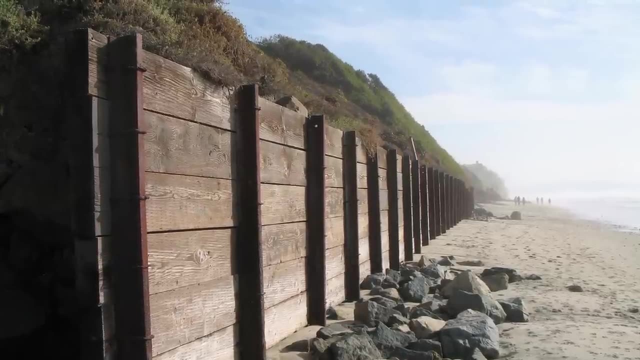 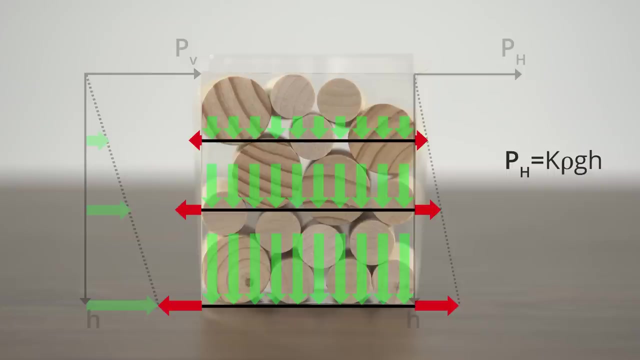 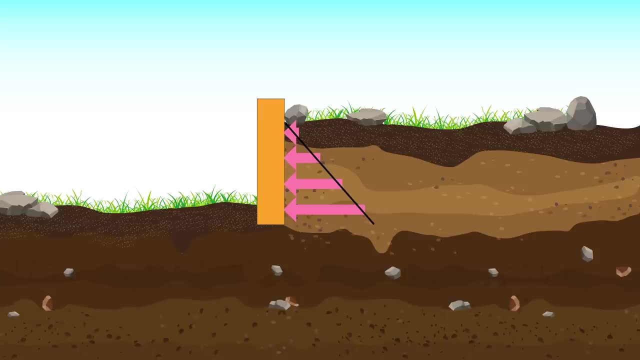 Retaining walls serve the important role of holding back soil and rock, just as dams hold back water. The first video in this series showed that granular materials such as soil and rock generate horizontal pressures that increase linearly with depth. Retaining walls must. 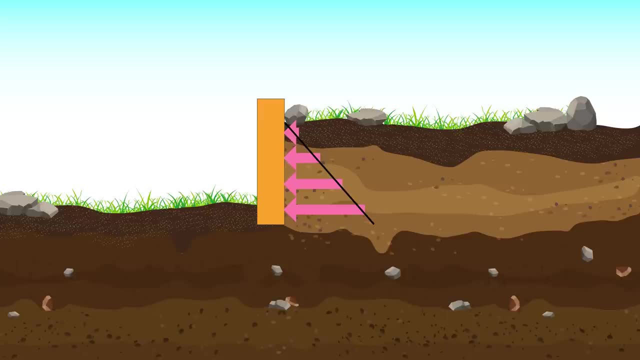 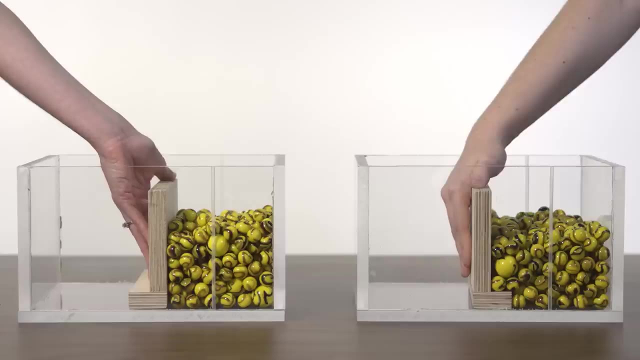 resist these pressures, and many strategies exist for doing so. In this video, we focus on the popular L-shaped cantilever design. If you were going to use an L-shaped wall to hold back soil and rock, as represented by these marbles, would you point the bottom leg towards the marbles or 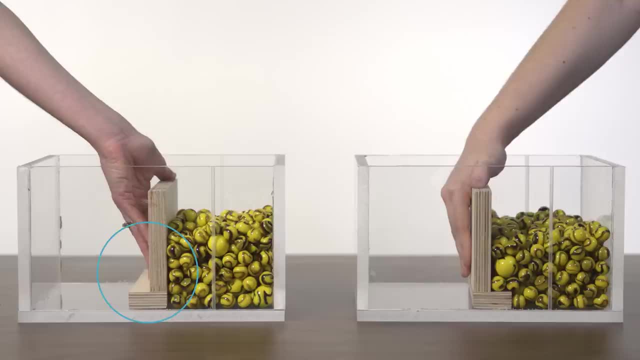 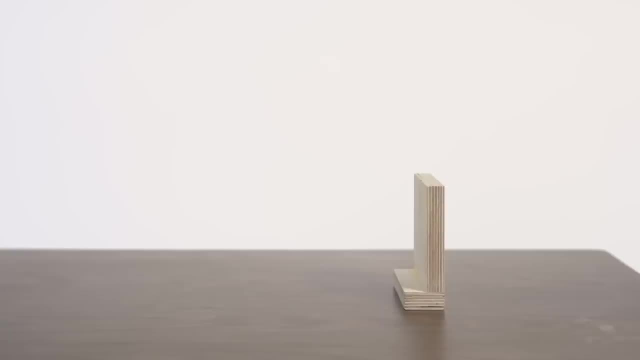 away from them. Many people would say that the base of the L should face away from the marbles. They probably realize that it is hard to tip the wall over towards the left if the bottom leg points in that direction. In engineering we call tipping like this overturning, If the bottom leg 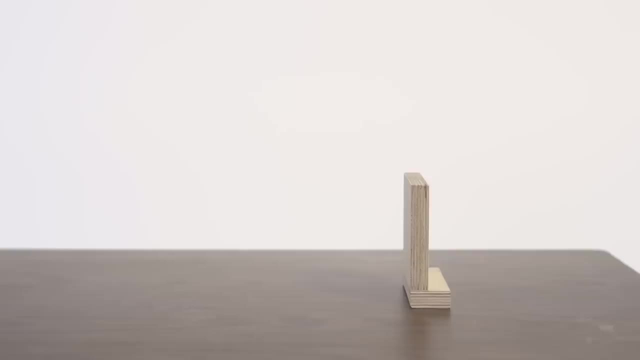 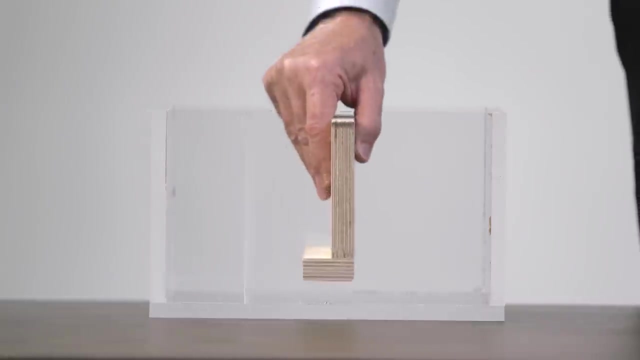 points the other way around. it is easy to make the wall overturn- So easy, in fact, that I can do it with just a puff of air. It looks like the case is closed, Or is it? Before we declare a final verdict, let's use the model to find out what happens when the bottom leg points to the left. 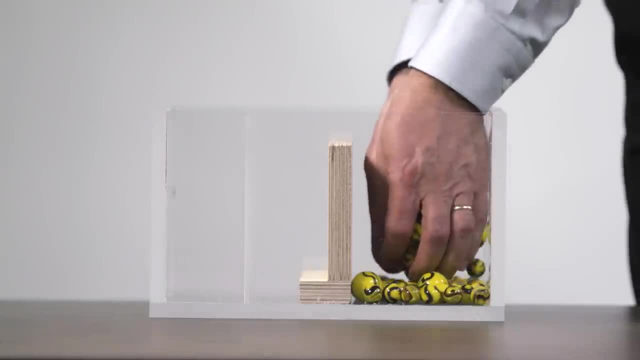 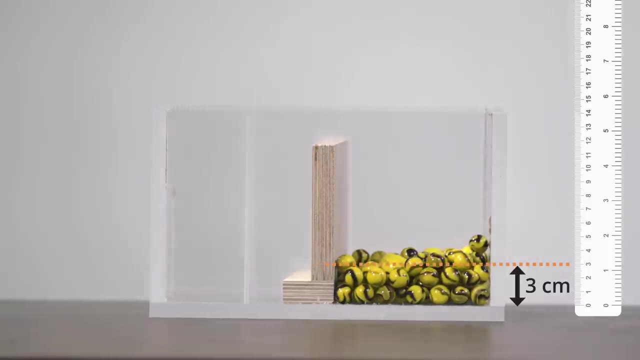 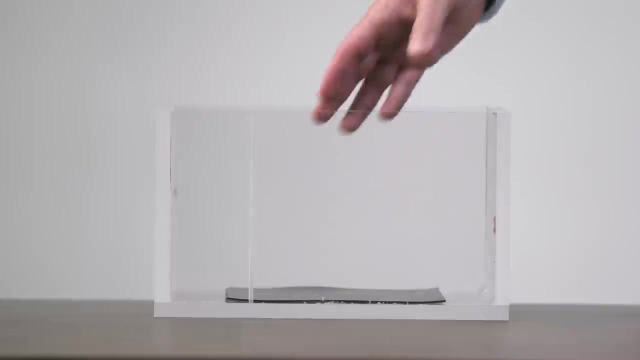 away from the marbles. As we add marbles, we discover that the horizontal forces they produce create yet another mode of failure, namely sliding of the wall, And this occurs when the marbles reach a depth of three centimeters. In the model, we can increase the friction between the retaining wall and the base by: 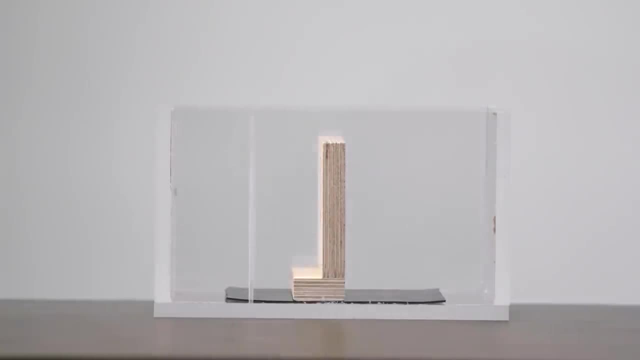 placing a rubber mat between them. You will have to do some extra reading if you want to find out how they achieve this end in the real world. As you can see, increasing the friction allows our model wall to support a noticeably greater depth of marbles. 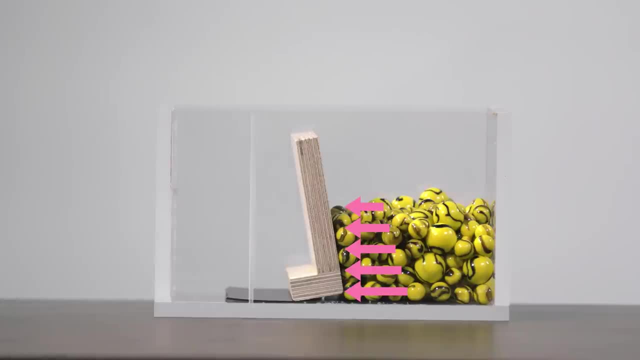 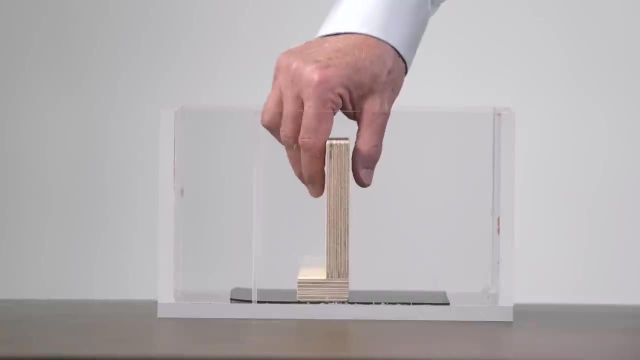 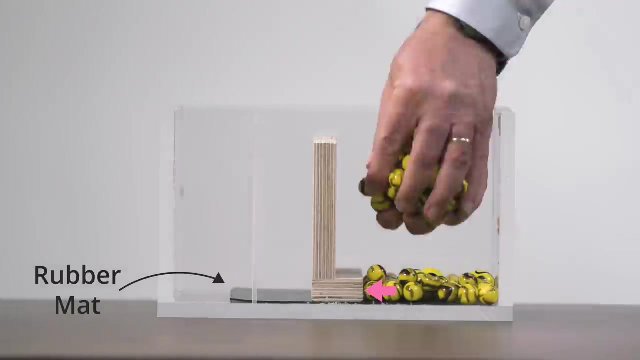 But it still eventually fails by overturning, in this case when the depth reaches eight centimeters. Now let's turn the wall around, so it's bottom leg points towards the right, The side where the marbles will be placed. We again use the rubber sheet to prevent sliding and we add some marbles as 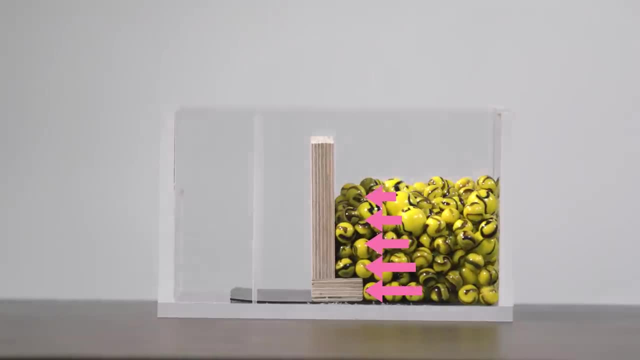 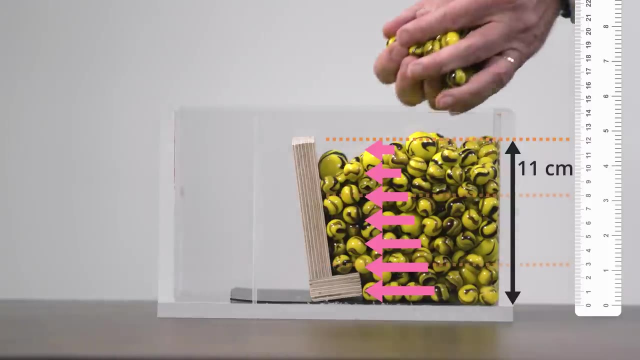 before the marbles generate a horizontal force that depends on the marble depth. You might be surprised that this wall can hold back eleven centimeters of marble marbles before it overturns. Can you explain why the wall can resist a greater height of marbles? 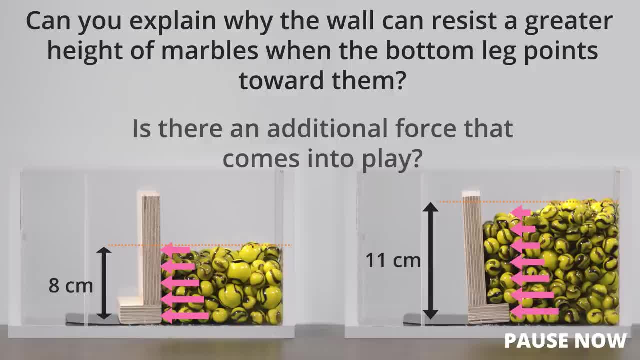 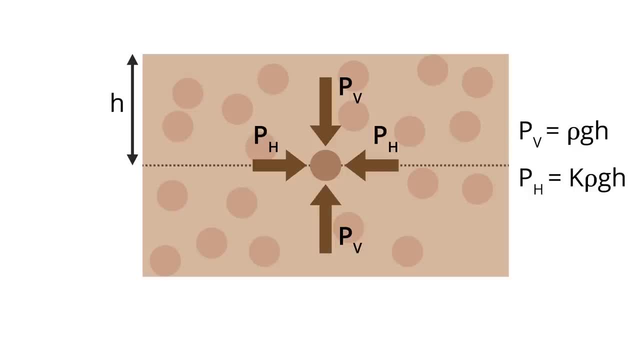 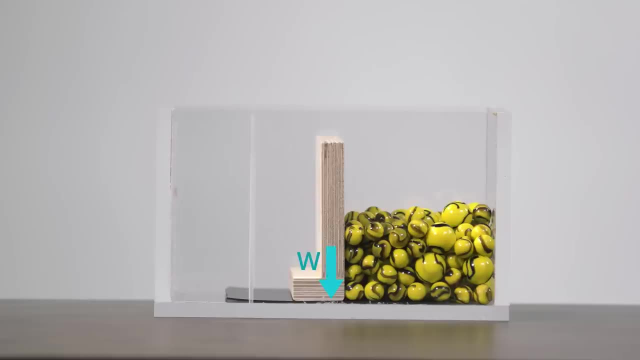 when the bottom leg points towards them, Is there an additional force that comes into play? Recall that granular materials generate both horizontal and vertical pressures. When the bottom leg is oriented away from the marbles, overturning is resisted only by the weight of the wall itself, and so it overturns easily When the bottom leg points towards the 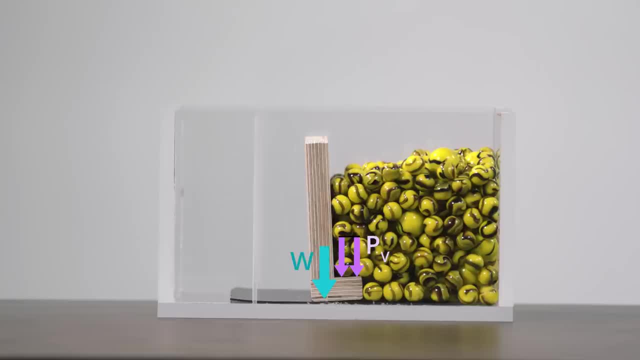 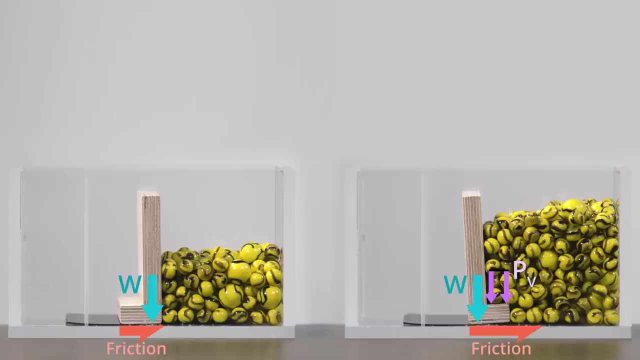 marbles. the vertical pressure from the marbles helps to keep the wall upright. The downward pressure also increases the friction between the bottom of the wall and the ground, thereby reducing the likelihood of sliding. When engineers design L-shaped retaining walls, they imagine them. 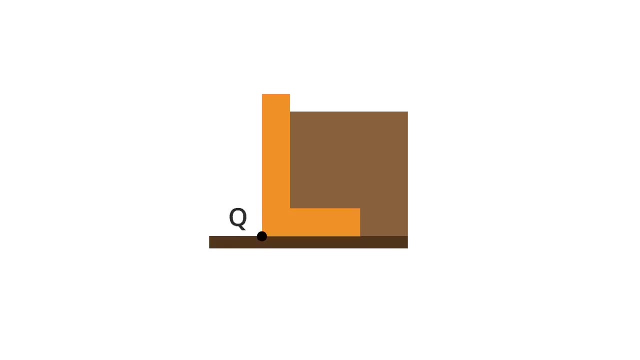 overturning. about the point labeled Q. They first calculate how strongly the soil pressure will tend to make the wall rotate. about Q, We call this tendency to tip an overturning moment and we label it M. Next they figure out the stabilizing moment MS, produced by the soil pushing downwards on. 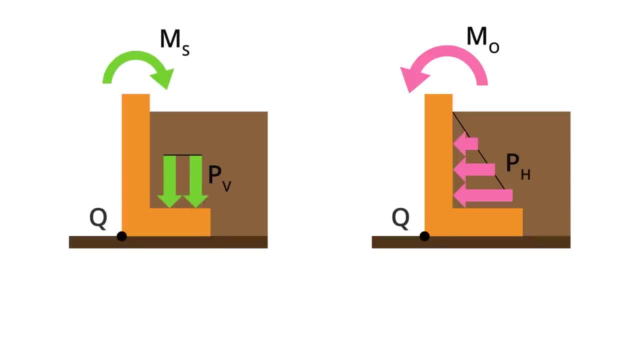 the horizontal leg of the wall. Lastly, they make sure that the horizontal leg is long enough that the stabilizing moment is at least as large as the overturning moment. Then the retaining wall will be stable. You might be surprised to learn that L-shaped. 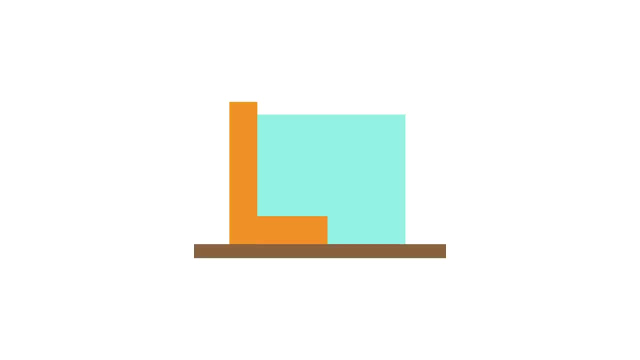 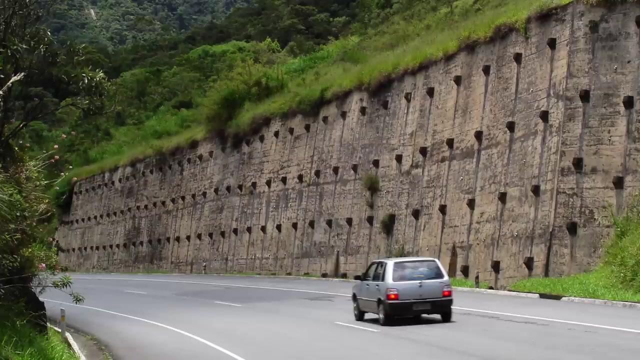 walls are seldom used as dams. The reason is that pressurized water at the bottom of the dam can keep under the base of the dam and if it does, the resulting upward water pressure on the bottom of the dam can generate an additional moment and make the dam overturn. Lots of other clever 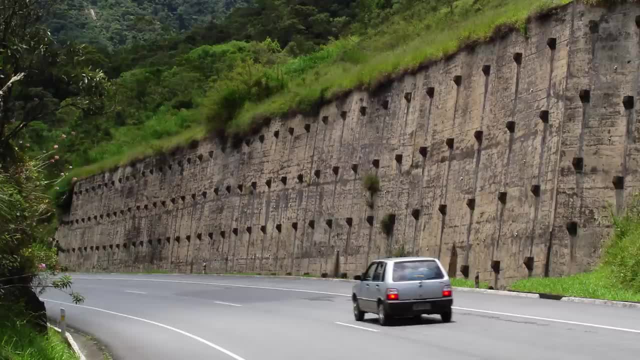 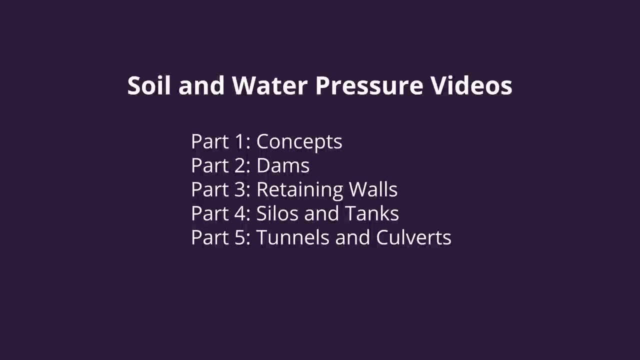 approaches can be used to design retaining walls, but we do not have time to discuss them here. To learn more about how soil, water and other materials interact with structures, we hope you will view our videos on dams, silos and tanks, and tunnels and culverts. Subtitles by the Amaraorg community.